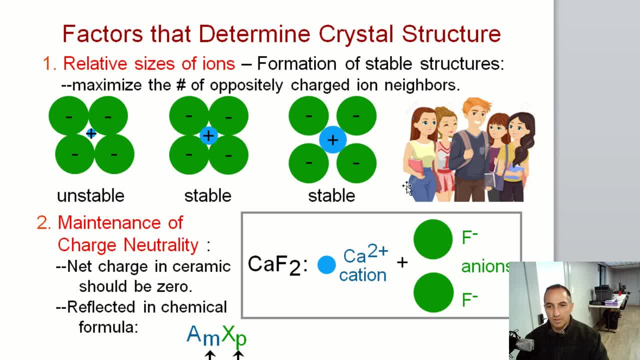 So as far as the distance between the atoms, you remember early on in the subject we showed an energy versus atomic distance between the atoms And there is a minimum energy where the distance between the atoms is stable. If they start to get too close to each other there is a very large repulsive force and the energy is very high because atoms separated. 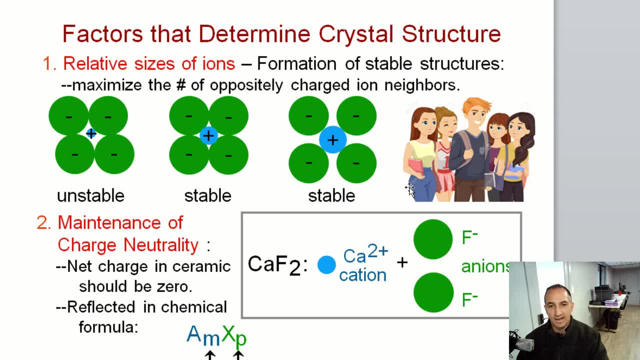 If they start to get too close to each other, there is a very large repulsive force and the energy is very high because atoms separated And also if you get further apart from the atoms then the energy goes up as well. So the minimum bonding energy has a stable point. 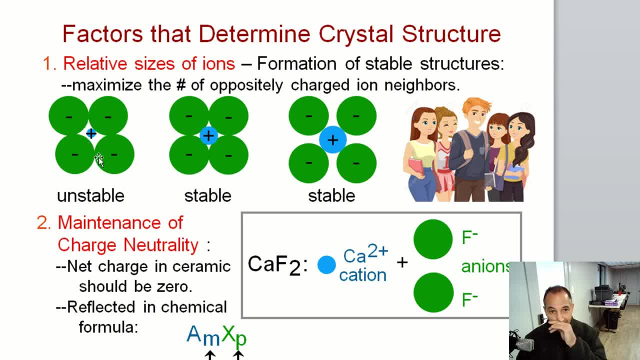 The common. The structure on the left here, where there is gaps between the cations and the anions, is not stable And on the right, two structures. you do have a stable structure there. The second is the maintenance of charge neutrality. So just to back up for a minute. I didn't mention the introduction of cations. 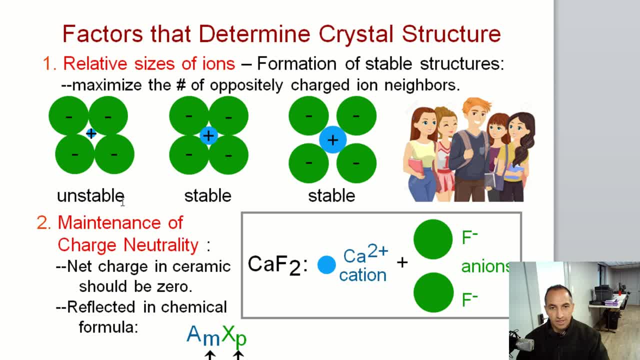 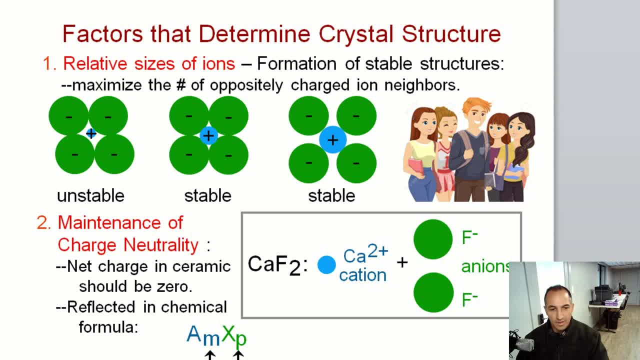 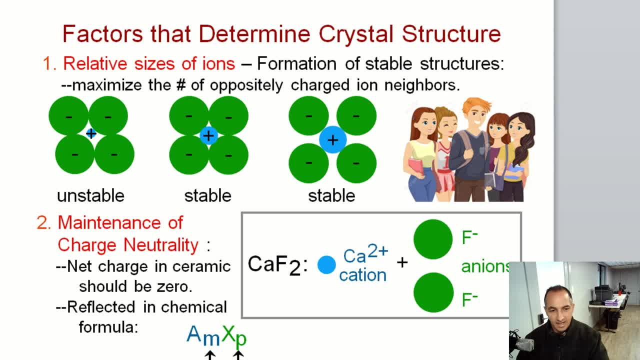 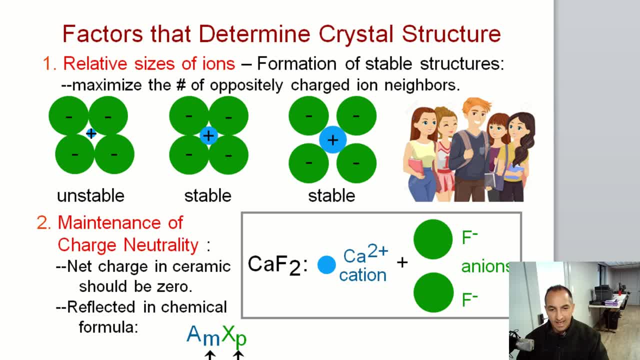 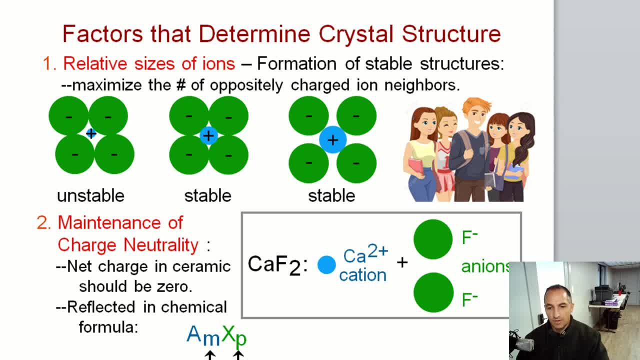 And the cations are always smaller than the anions And the cations are always smaller than the anions And the cations are always smaller than the anions. And the reason why is because the cations give up electrons. And the reason why is because the cations give up electrons. 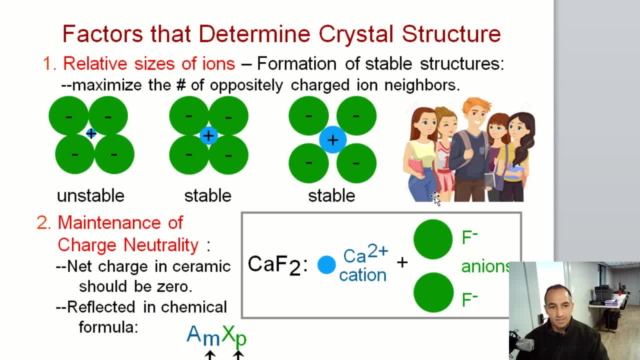 And when it becomes ionized. so the remaining electrons are held more closely. And the reason why is because the cations give up electrons. And the reason why is because the cations give up electrons. And the reason why is because the cations give up electrons. 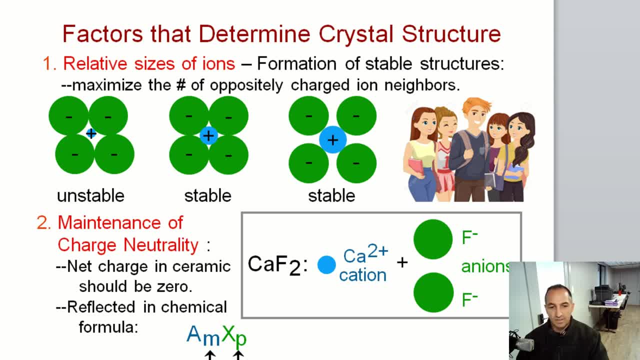 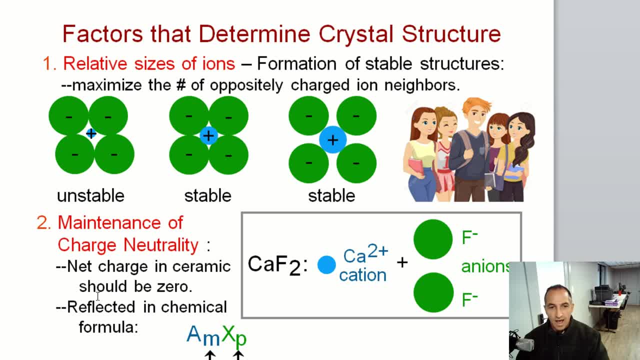 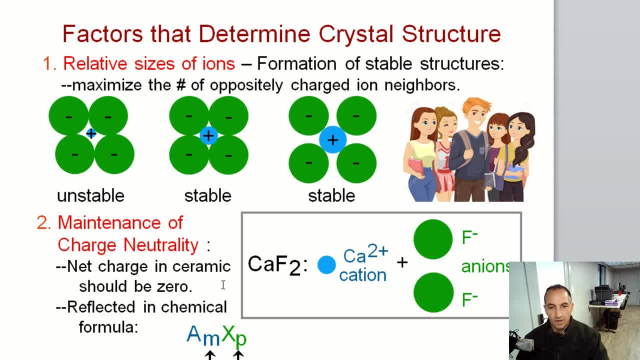 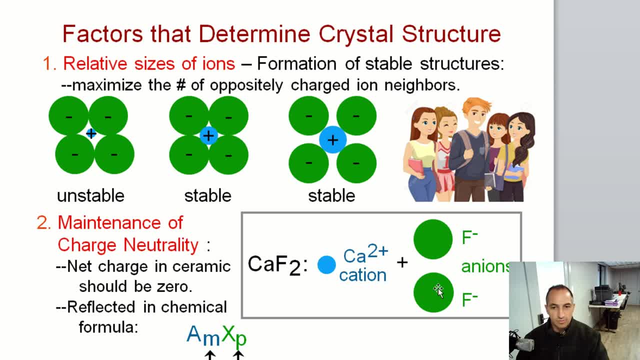 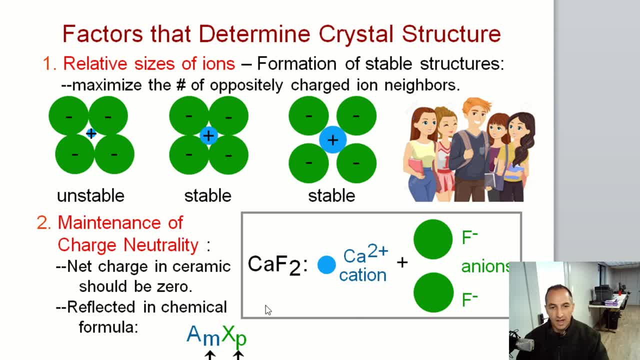 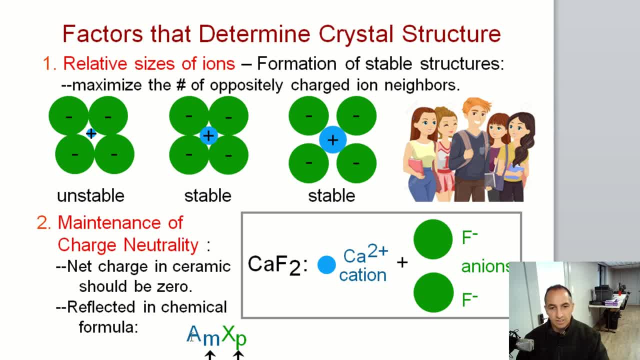 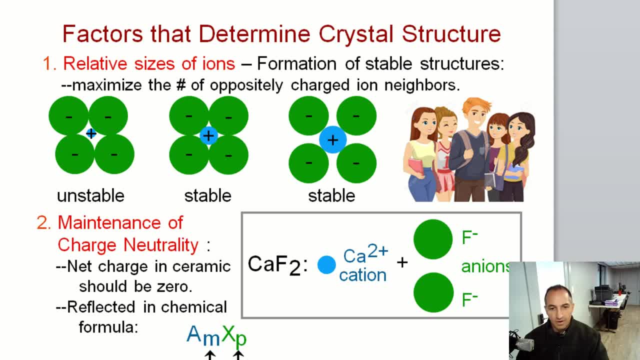 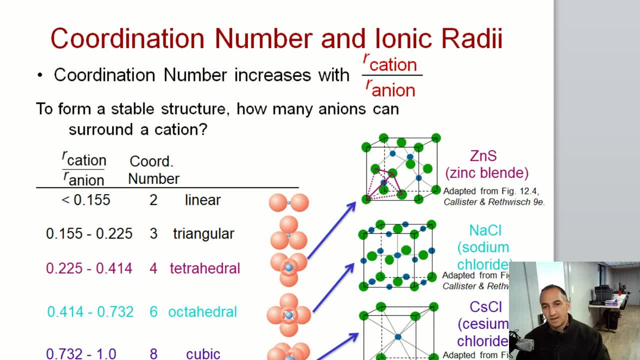 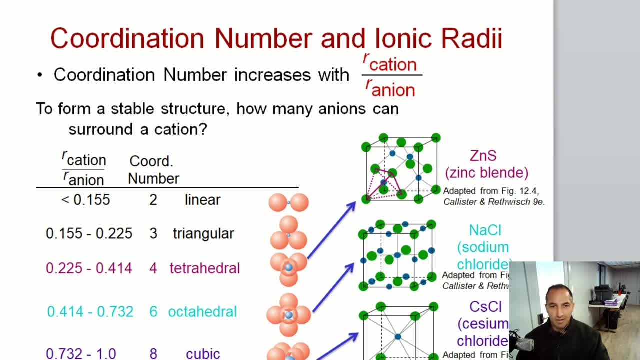 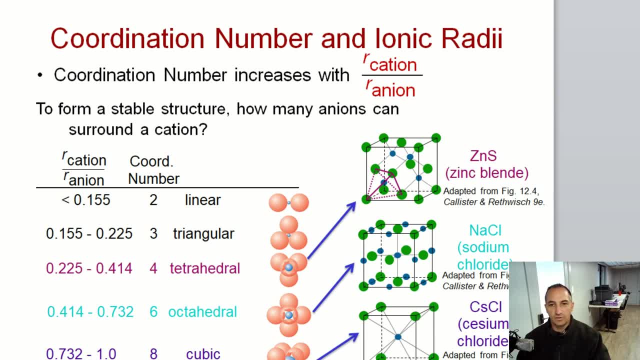 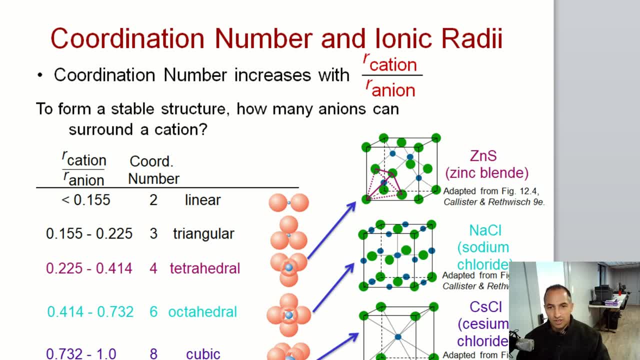 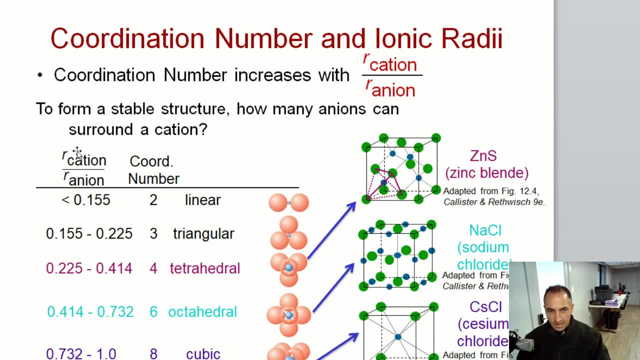 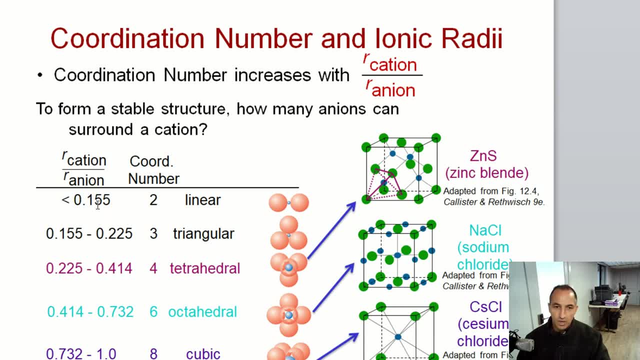 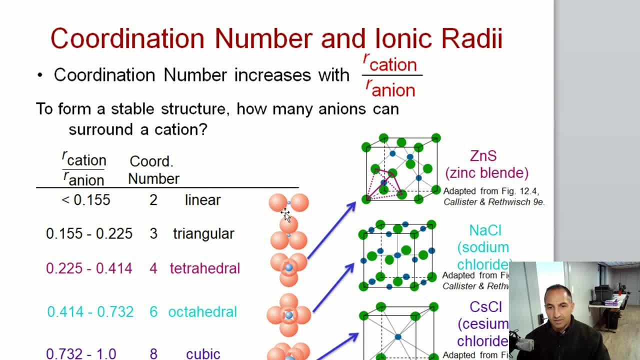 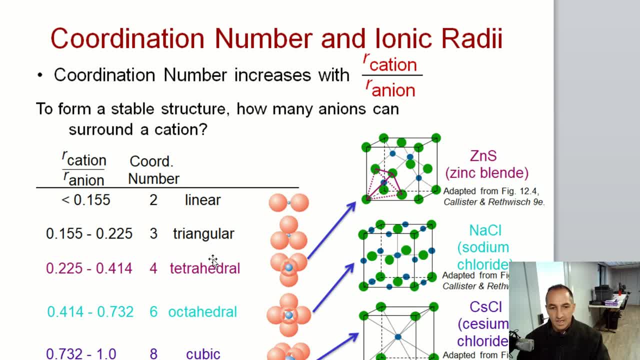 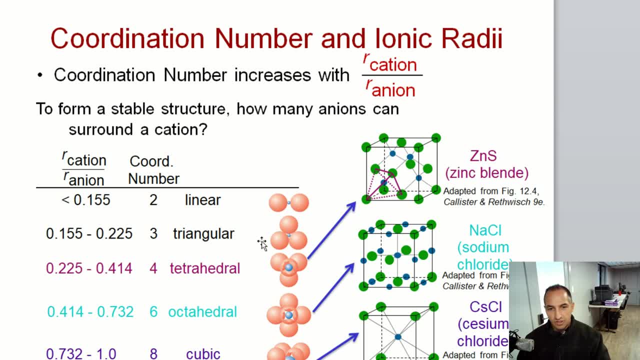 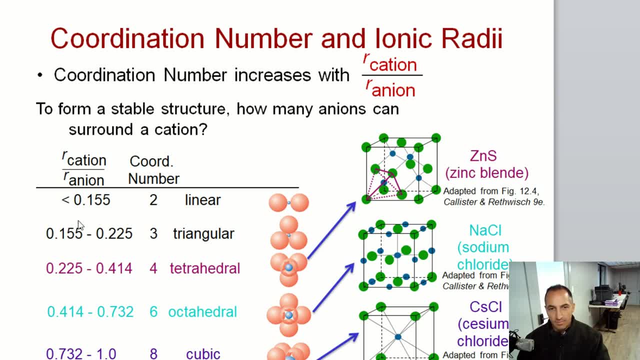 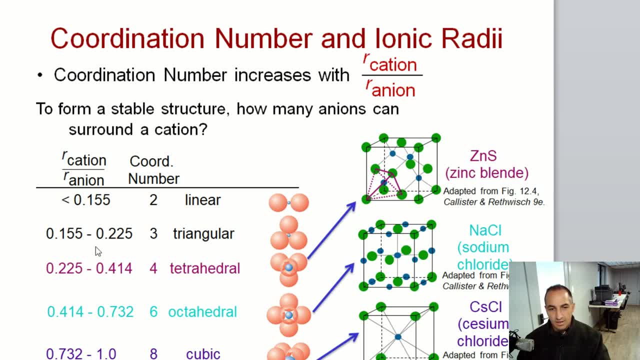 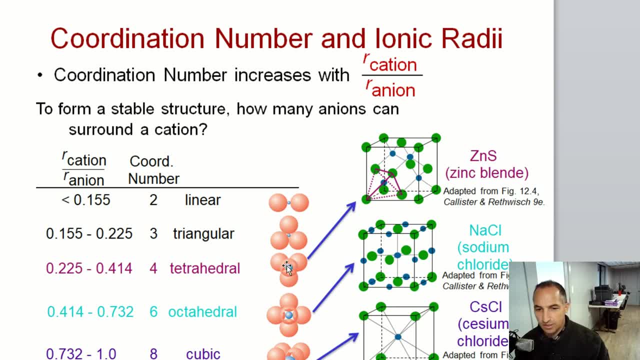 more and more anions surrounding the cation, so the coordination number of four, or the tetrahedral. that's a very common crystal structure and that's also called the zinc blend or zinc sulfide crystal structure. we're gonna go into each of these a little bit more on the following slides. so then the octahedral. 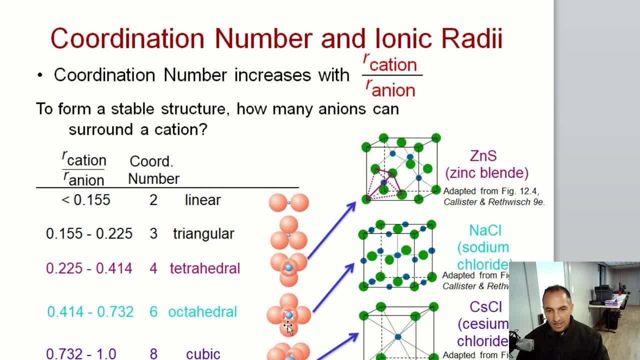 has a coordination number of six, as you can see here. there's the four surrounding, plus one on top, one on bottom, and that is sodium chloride crystal structure and finally the cubic crystal structure, also called the cesium chloride structure. it looks like the one here to the right. 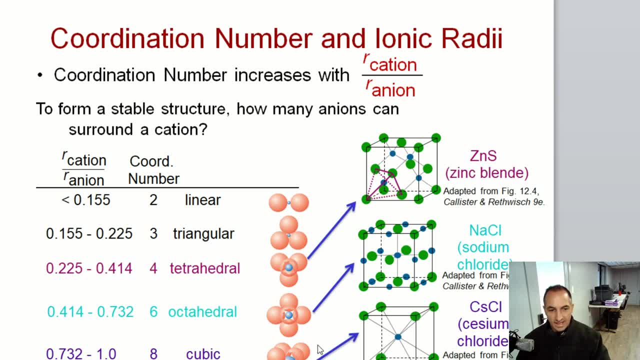 so as the cation gets bigger, point occurs when the cation gets bigger. the point occurs when the cation gets bigger, when they can be surrounded by another anion, and so that's what is going to happen there. so, going up here, we have larger and larger adion radiuses going. 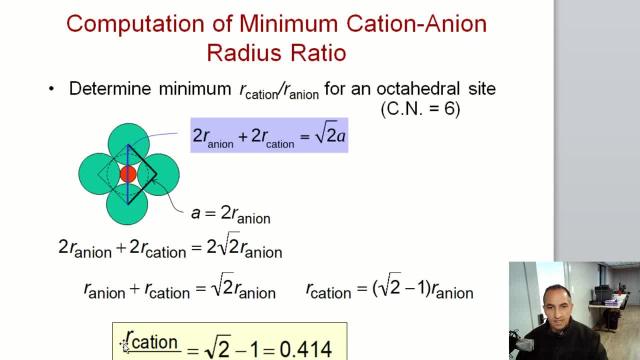 from top to bottom, though its geometry here determines what that adion to ion ratio is for each of the types of crystal cations, and they are just shown here. also. we can see here that the crystal structures. So let's look at as an example the octahedral structure, which is the 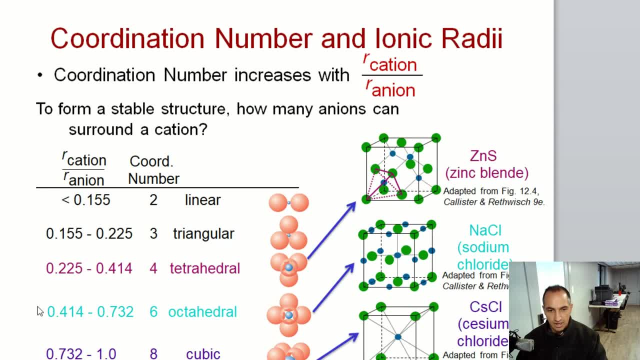 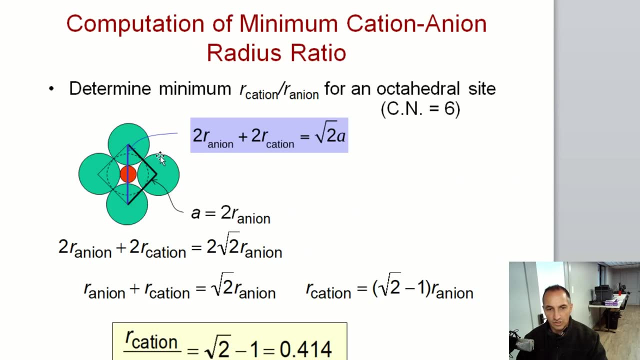 coordination number of six. So that's that, this one right here, So that you can see it has the four surrounding, plus one on top, one on bottom. So this is a slice looking- sorry, this is a slice looking straight down- at those four anions surrounding the one cation here, which is the. 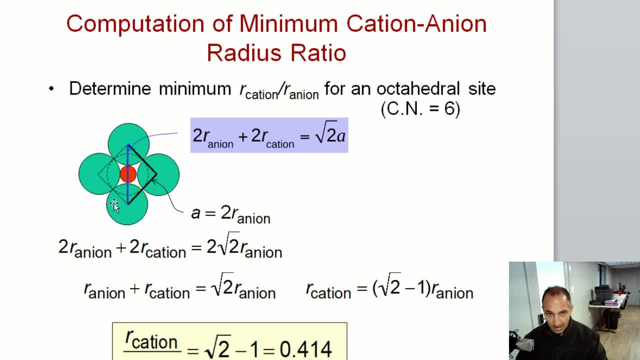 red one in the middle And the dotted line is the anion that's directly above and another anion that's directly below this. So to determine the ratio of the cation to anion, we have to first look at the relationship to A, which is: 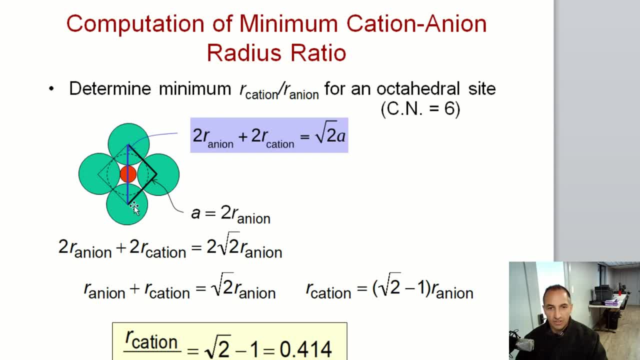 the unit cell length for this octahedral. And the unit cell length is just A here. So that is also equal to two of the anion radiuses. We've got one radius here and one radius here. Additionally we can determine the length of the diagonal of this 45-45-90 triangle, which is: this is A, then the 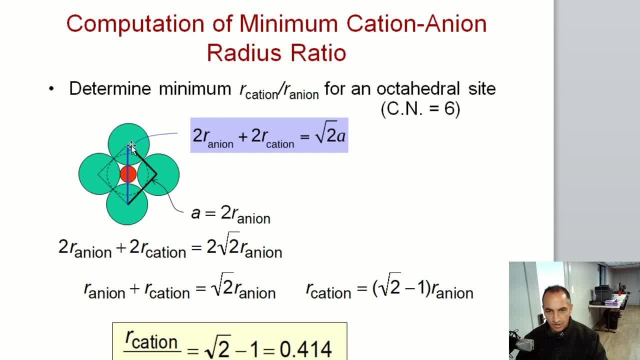 diagonal is 45-45-90.. So we can determine the length of the diagonal of this 45-45-90 triangle, which is root 2A, and that's also equal to two of the anion radiuses. We've got one here and one here. 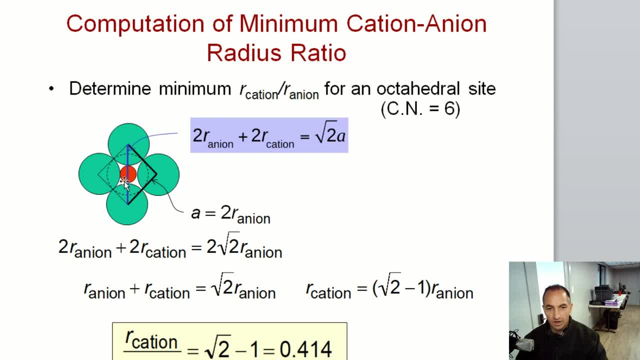 plus two of the cation ratios or radiuses. So there's two of the anions, two of the cations. Add those together that's equal in relationship to the unit cell length A. so that's equal to root 2A. So plugging. 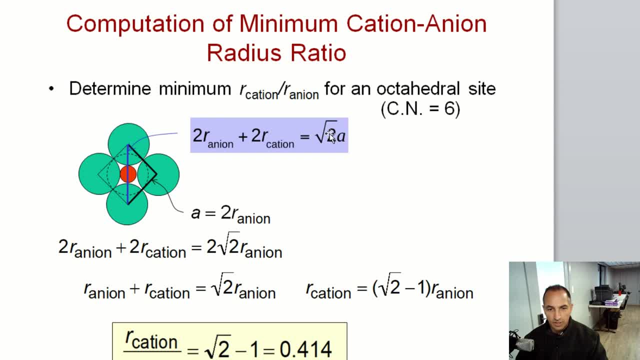 then in the root 2A- sorry, plugging in this into this equation here- then we get 2 root 2 times the radius of the anion, So simplifying this. then we just divide through by two, then this equation, then we isolate the. 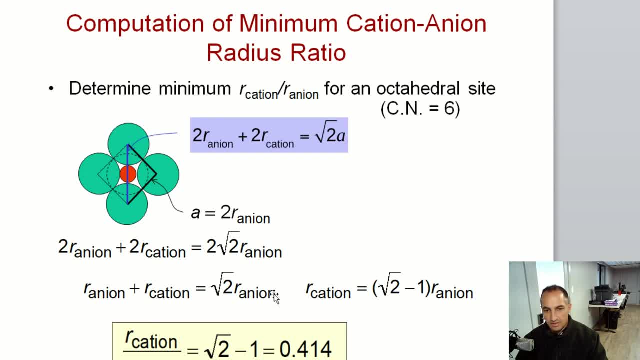 radius of the cation by subtracting the radius of the anion, So that's equal in relationship to the unit cell length. So we have the radius of the anion by both sides. and then factoring out the r-anion gives you then this equation here: 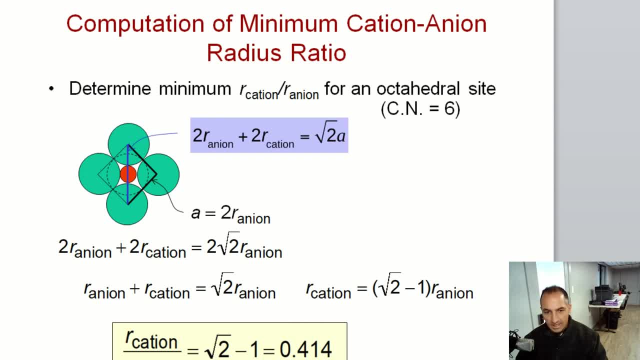 Then just dividing through again by the radius of the anion- both sides here- that then is equal to the root 2 minus 1, or 0.414.. So that number then is the minimum in the range for the octahedral. 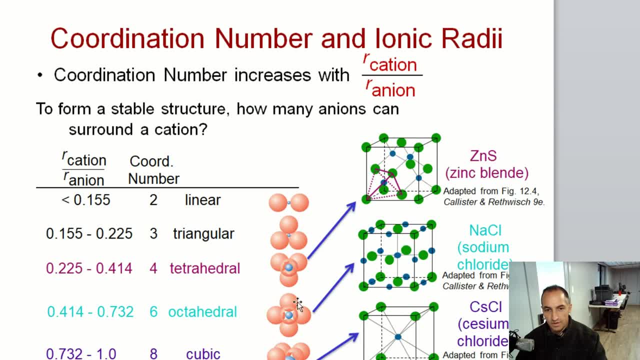 So that number then is the minimum in the range for the octahedral. So if you go back, look at 0.414,. if you go back here again the octahedral, the minimum for that range is 0.414.. 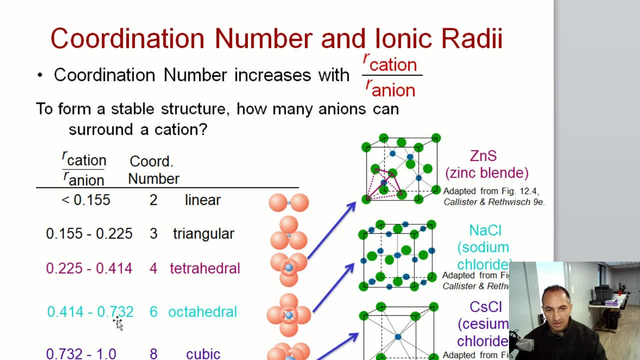 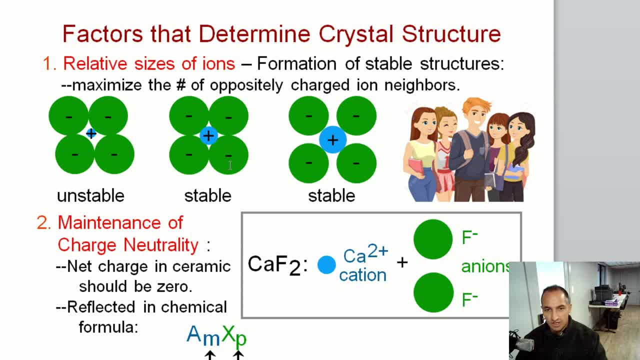 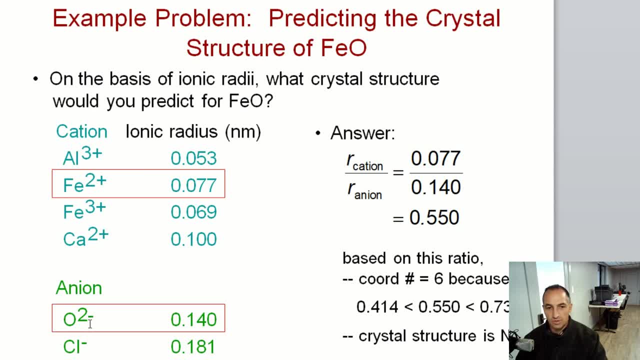 So if you go back to this slide, that's kind of what's going on here- where the minimum is the center image, oxygen is always a two minus. so because iron can take on a two plus or a three plus, we're going to select the two plus because that's what we recharge: neutrality and so the ratios of 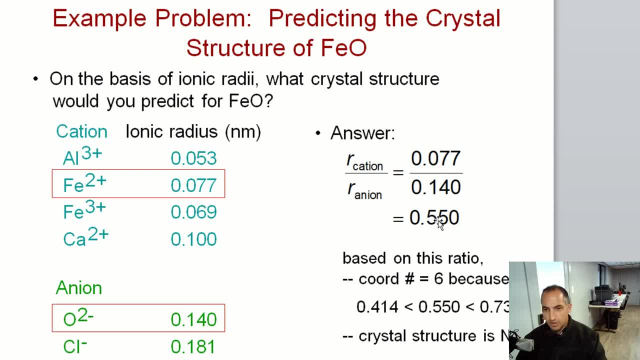 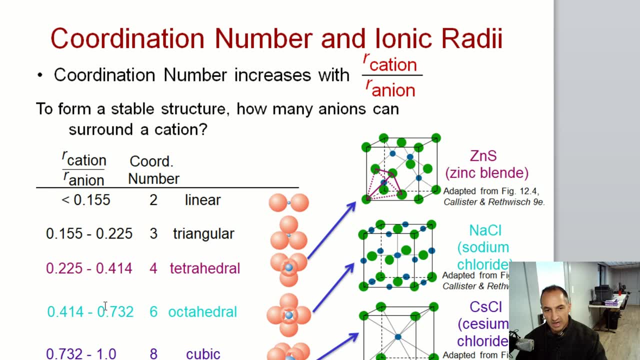 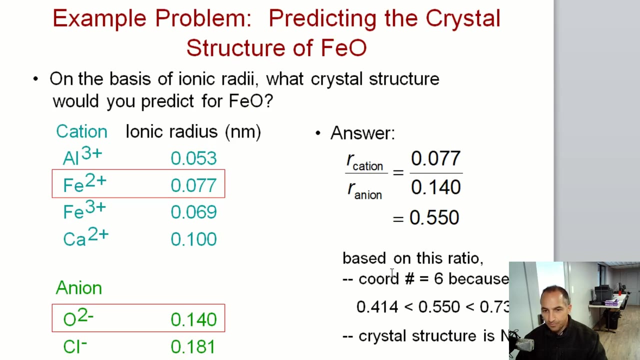 those two is then 0.55. so, going back to our table, where does 0.55 lies? well, it lies right in between this range here. so it would be a octahedral type or a sodium chloride type of crystal structure with a coordination number of six, and that's exactly what we have here, coordination number. 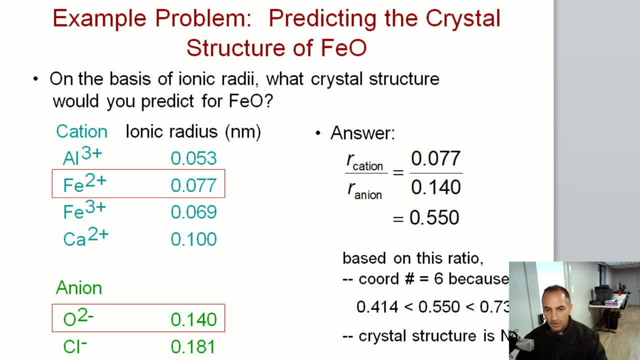 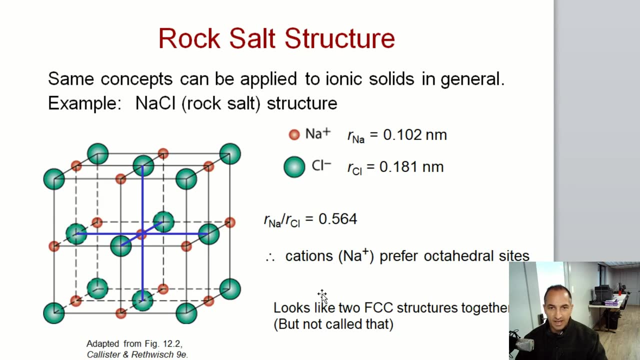 of six, and so it has the sodium chloride crystal structure. so you might be asking: why do we call it a sodium chloride crystals, when it's an actually an iron oxide? well, that is because we- I think it was because they first determined this type of octahedral structure with sodium chloride, and so just to give it a name. 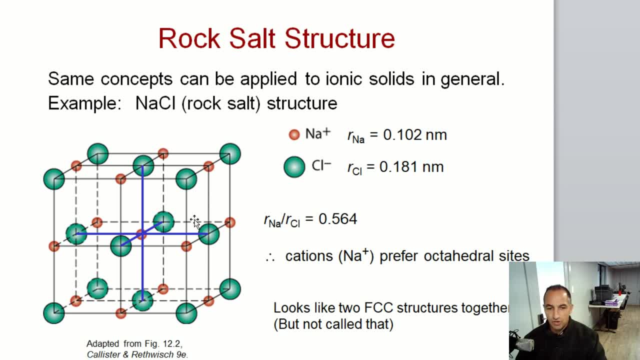 he called it the sodium chloride crystal structure, and so there are many other types of ceramics, though, that take on that rock-solid structure, and, for example, magnesium oxide or iron oxide, and if you look at a little bit more closely here, it's actually two interlocking FCC structures, if you just 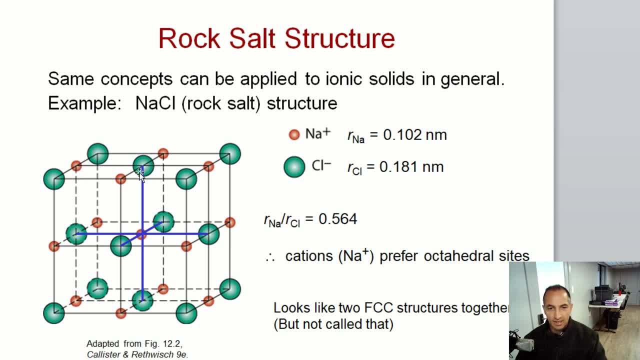 ignore the red cations here. just look at the fluorines. there's your familiar FCC structure. and if you just ignore the red cations here, just look at the fluorines- there's your familiar FCC, where you have four on the faces and then you have eight on the corner. 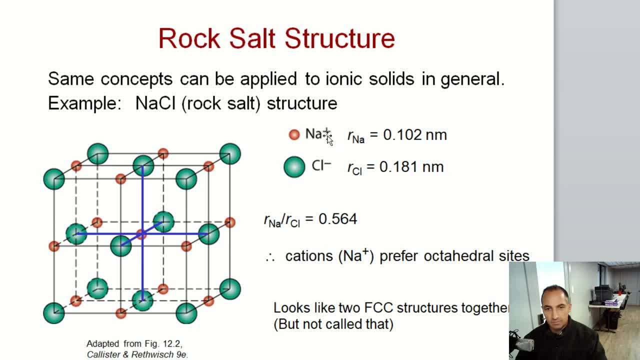 and then if you look at the sodium, then it's just shifted down by a half a unit cell length. so now these reds are the cornered atoms, and then these red ones down here are the base ones, and then you would have another set of quarter sodium. 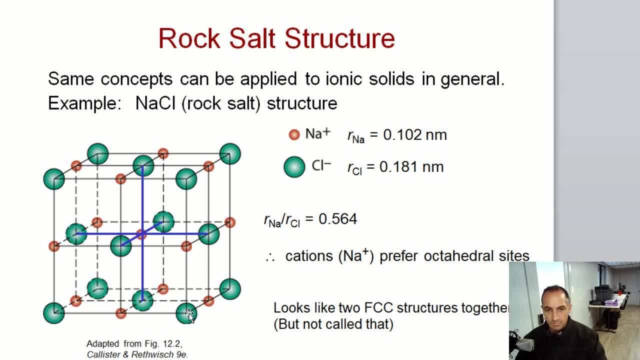 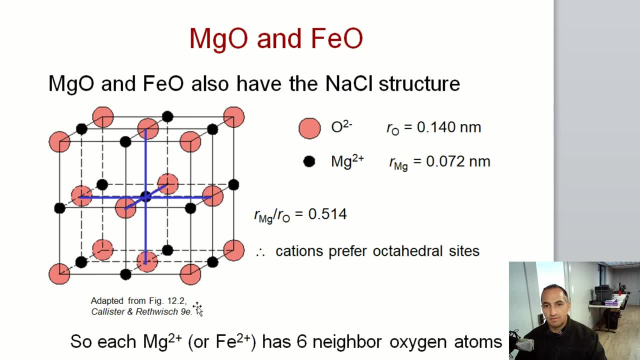 so on the bottom. so that's your two interlocking FCC structures, and I said that other types of sodium chloride or rock salt structures are dim oxide, iron oxide- here you have magnesium oxide and identical the previous one. it's just types of atoms and a slightly different ratio point. 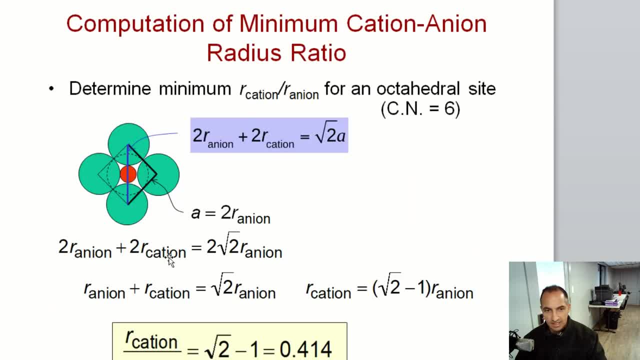 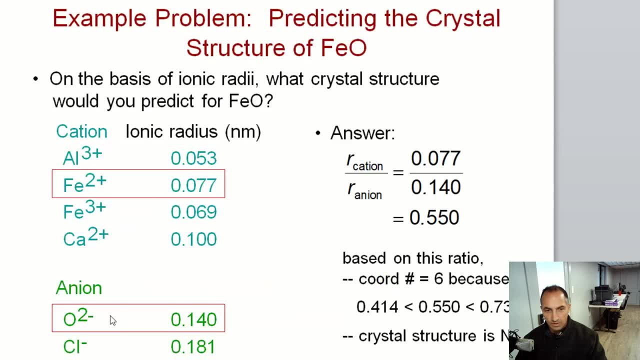 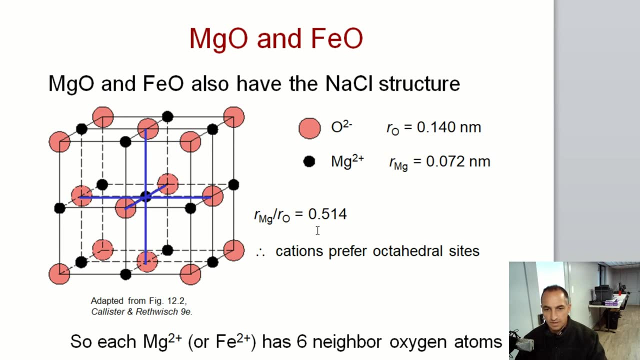 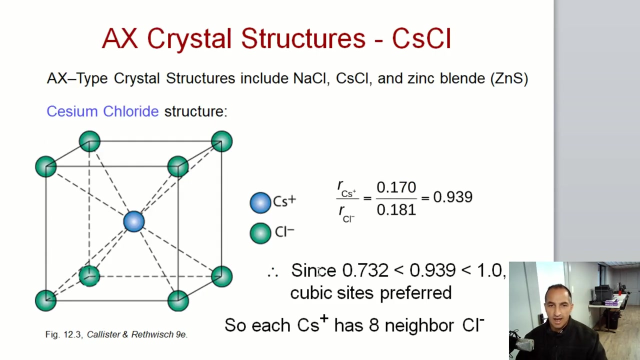 five, one, four. however, it still falls in that range. here in the rock salt, or sodium chloride structure still falls in that range. or magnesium oxide, and again with six nearest neighbors, now another type of crystal structure, and this is another ax. so that means that there's one anion for every one cation, at one to one ratio, just like the rock salt is ax. 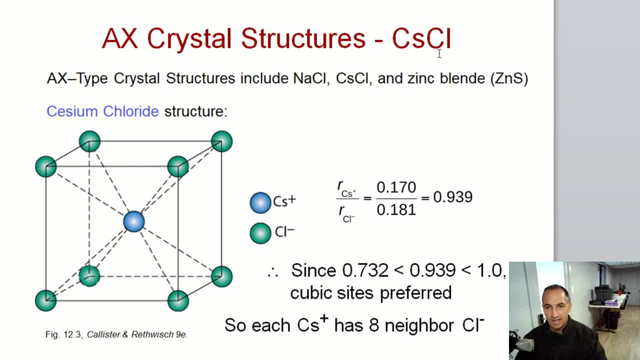 so, and this is called the cesium chloride crystal structure, and so with cesium chloride, differences in the anion to cation ratios is very much higher. so that means you can accommodate more anions around the cation 0.939 for this one that falls in. 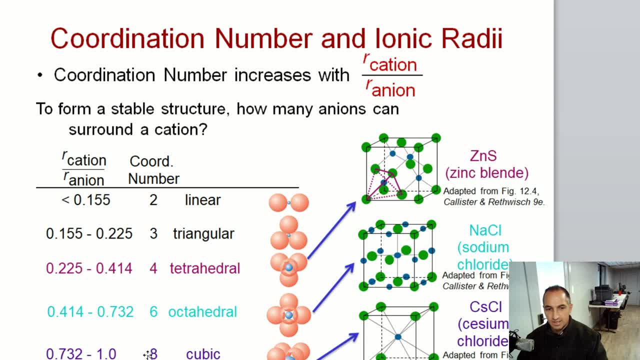 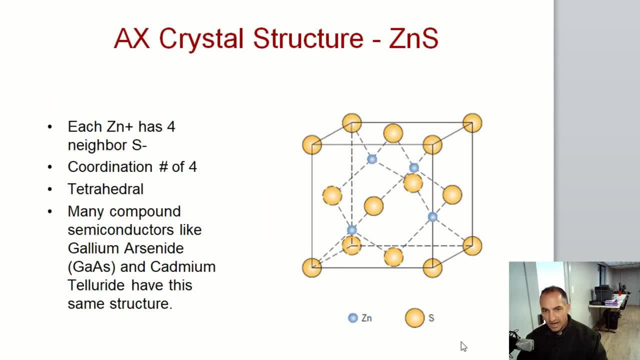 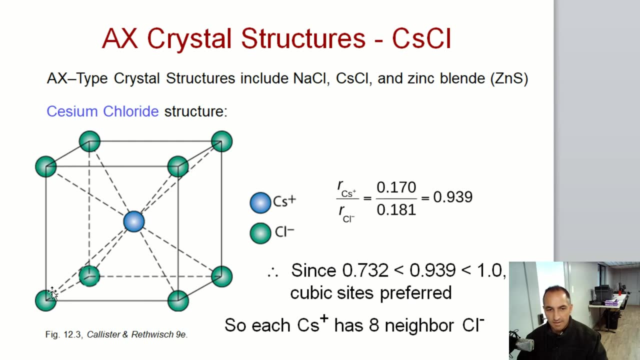 this range here with a coordination number of eight, and so that's that cesium chloride crystal structure. the cesium chloride has that eight. see how there's four nearest neighbors on top, four nearest neighbors on the bottom and it comes off at about one and a half, and then there's four nearest neighbors on the bottom. 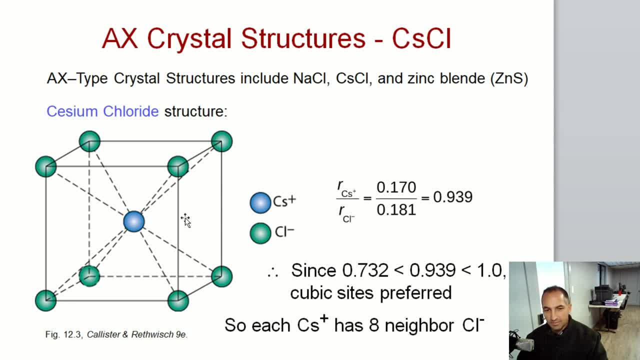 here. so that's a nice square box into the and it looks kind of like bcc if you take both atoms together. but as we have two, look at each anti-insane separately it's more like a simple cubic, or the or the chlorine, and that's why it's called. 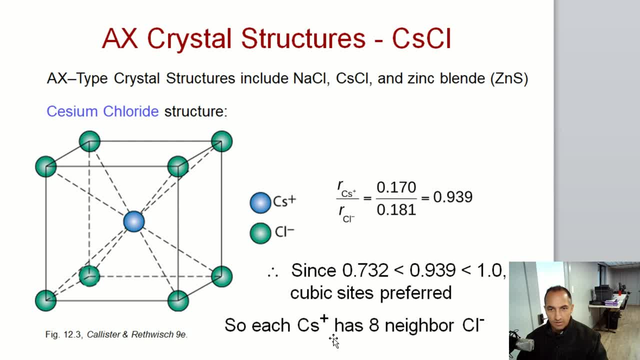 the cubic structure. so, and that's a cesium chloride. so this is called a cesium chloride crystal. so it's a, a black bcc crystal. so that's why it's a cesium chloride crystal. so that's a bcc crystal. so that's why it's called a. 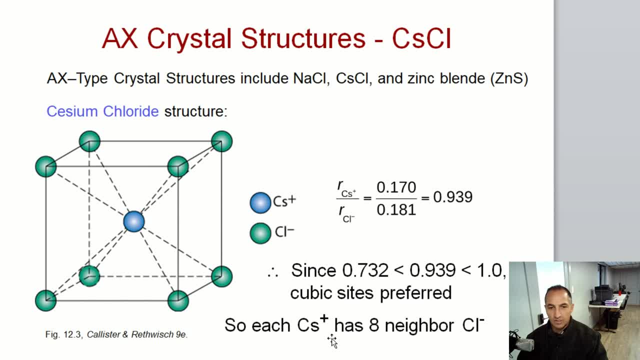 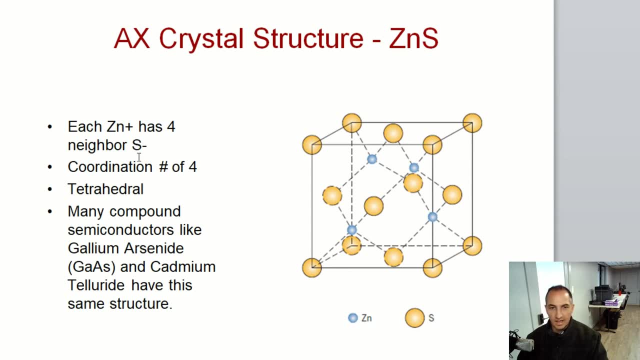 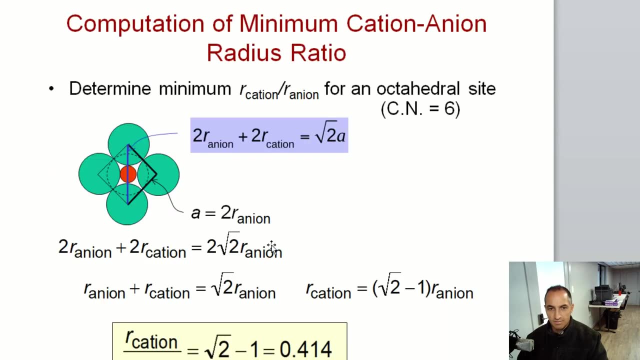 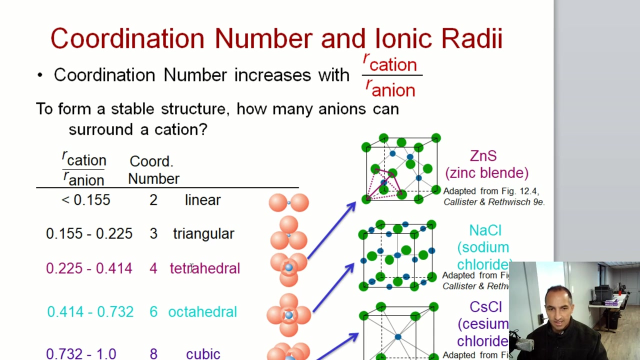 fluoride. so there are other types of cesium fluoride structures and but this one is the, the other type which is called the zinc sulfide or zinc blend, kind of jumping around from here, remember. okay, so zinc blend is this one right here. zinc blend as a coordination number four, and it's in the range in: 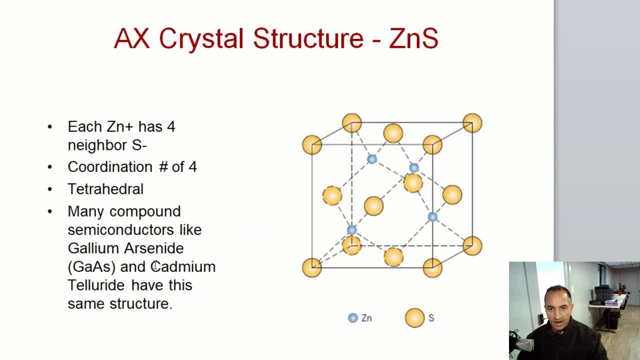 this range here. so, going back over to the, the zinc blend, or example of this is zinc sulfide. and if we look at other types of compounds, semiconductor compounds like gallium arsenide, just a compound semiconductor, I mean telluride and the. these are not technically ceramics but we borrow the structure, the ceramic. 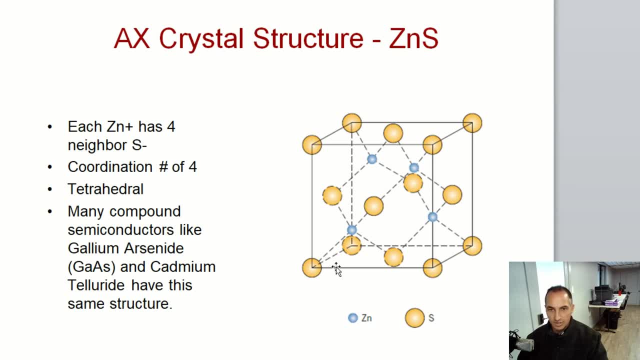 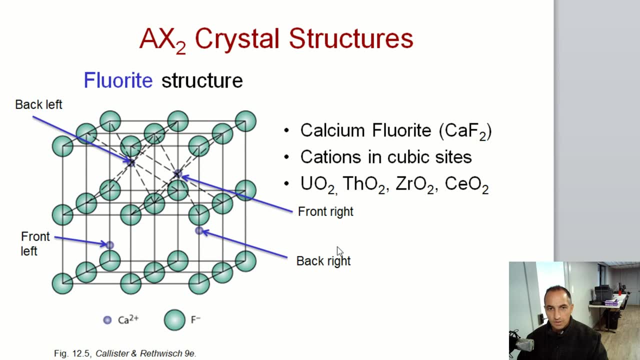 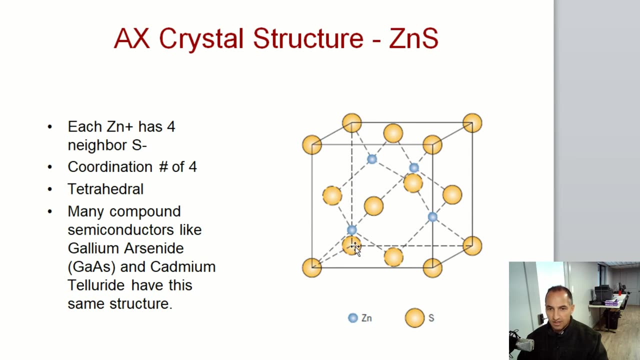 structure name for these compound semiconductors. so we do call those zinc blend semiconductors. so, looking at that, alright, I jumped forward alright. so there is what it looks like. you have these zinc atoms lattice of, like tetrahedrons, and so you have, like you know, four when one, two. 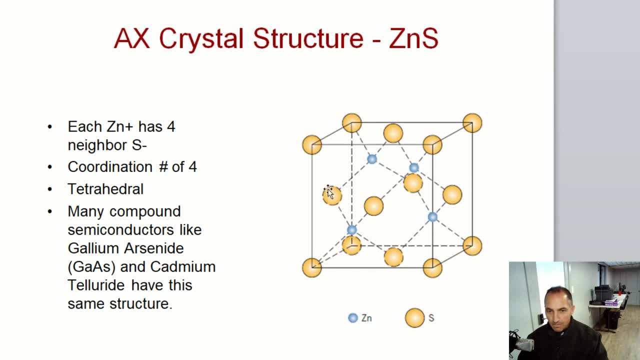 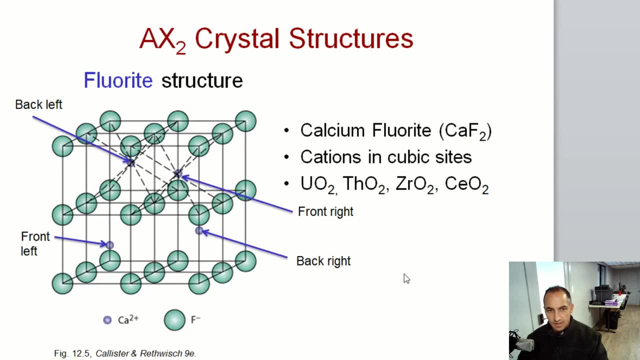 three, four nearest anions for each of these zinc. all right, so let's look at the um, the fluoride structure of the zinc blend, and we're going to look at the fluoride structure of the zinc blend. and we're going to look at the fluoride. this is the ax2 crystal structure, meaning there's two fluorines for each of the. 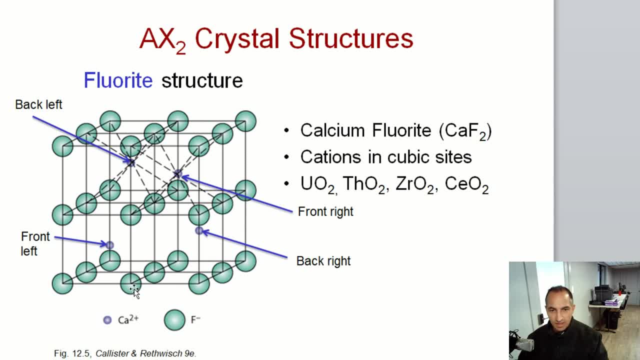 calcium, and this is a little bit harder to visualize. so this actually has eight cubic structures, whoa, eight cubic structures here: one, two, three, four, five, six, seven, eight. the cubics are the chlorine atoms. so there has to be twice as many chlorine atoms here as the as the calcium and the calcium's are going to try to be as far. 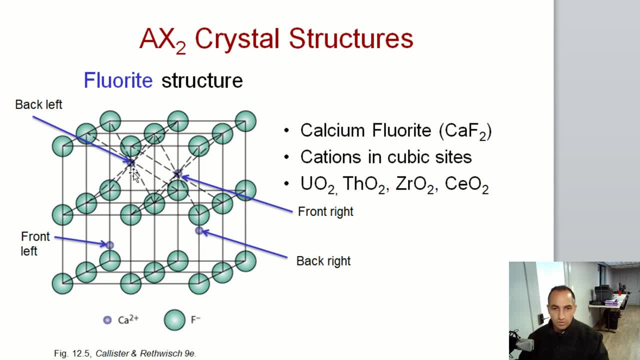 away from each other as possible. so to do that for the calcium's being in the interstitial sites, this calcium then is in our left back cube, and then the next one to get the spacing far away from each other is going to be in the front. 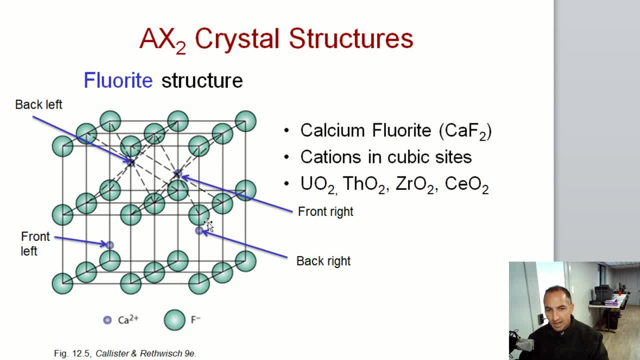 right, Q, and in order for then that the other two calcium's to be as far away from the top two, then they take the alternating sites, interstitial sites, site. so this calcium is going to be in the back right and then this calcium is going to be in the front left, so this one's in the back, this one's in the. 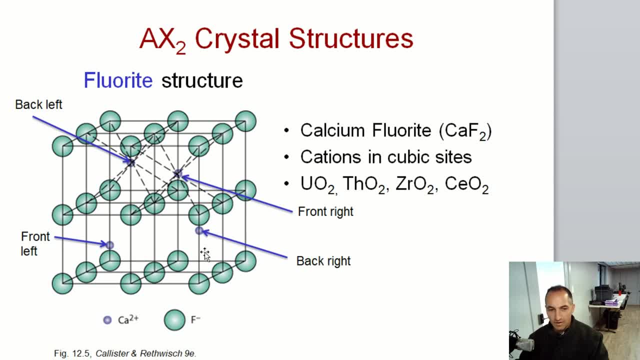 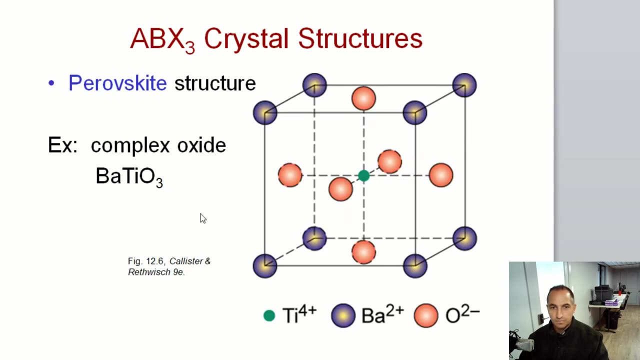 front. this one's in the front, it's with the back being as far away from each other as possible, and they're going to occupy the center of the cubes, the interstitial sites of this. all right, so that's the fluorite structure. another type of crystal structure is the perovskite structure. this is actually a 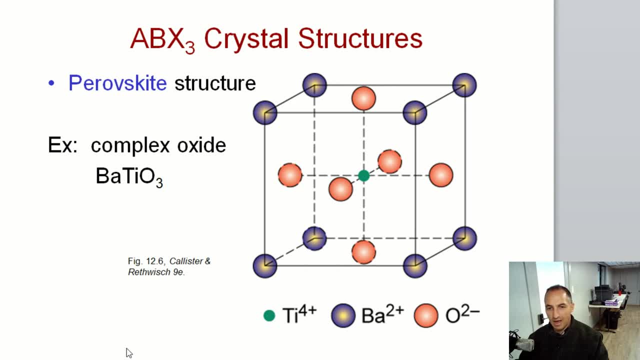 type of ceramic that's really increasing in popularity now. after spending so much time in the research labs- and this one is a strong material for me because I studied it as a graduate student- use in non-volatile memories applications, and what you have here is titanium, which is this small ion that's 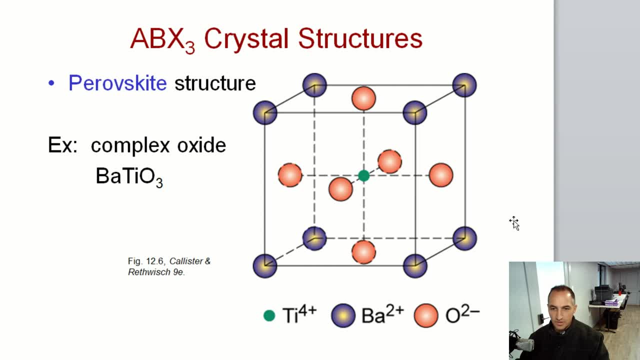 in the center, and then you have the barium which are on the corners and the oxygens which are on the faces, and this, this titanium, doesn't always want to be right at the center, either is offset above or offset below a little bit. that's where it it maintains the furthest separation from. 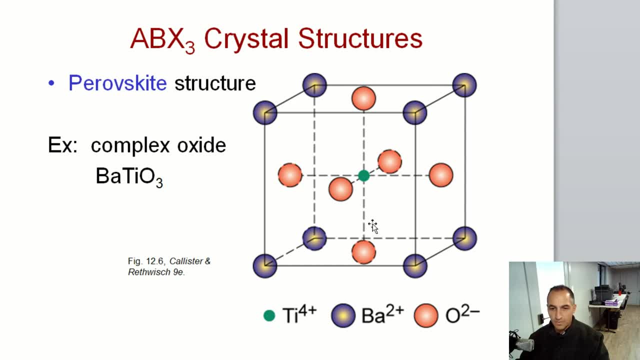 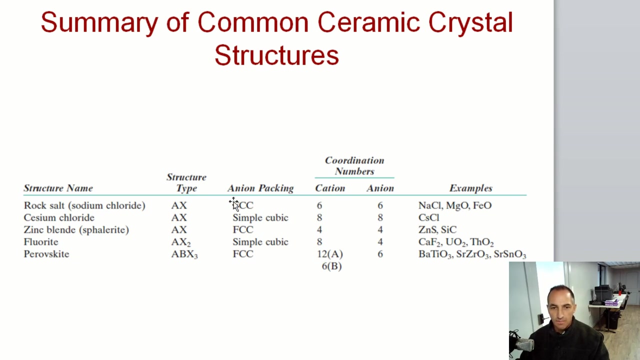 the other atoms in this cube. so that's why it's considered a ferroelectric and it's also increasing popularity now as a high-efficiency solar cell material. so in summary, of a common crystal structures we have the rock salt sodium chloride. structure type is AX, cesium chloride also. 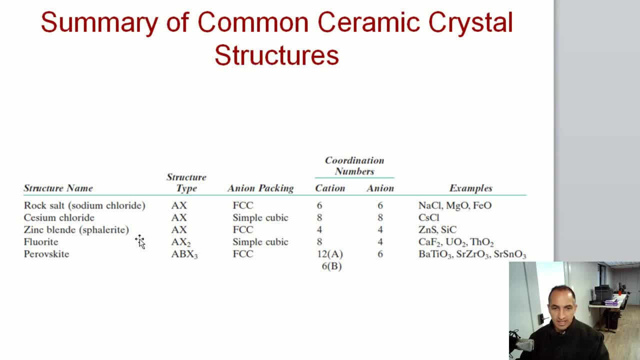 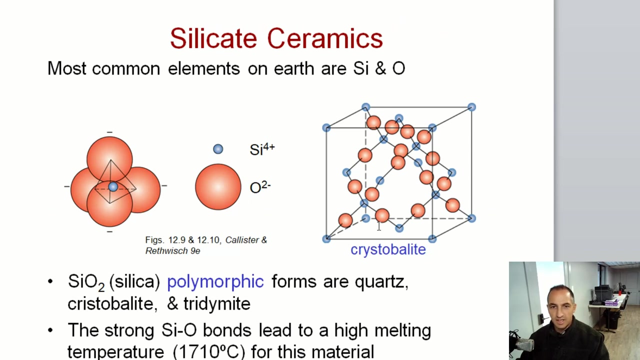 AX and the zinc blend is also AX and the fluorite is AX2 and perovskite is ABX3, and here are some examples of each of those here and their coordination numbers. so, skipping gears a little bit, now we're going to jump into silicate ceramics, so 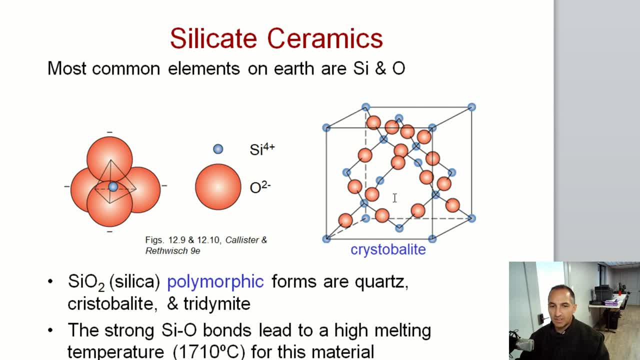 silicon oxygen are the most common elements on earth. so here is the Sio2, which is also called silica. its polymorphic. polymorphic form can be either quartz, cristobalite or tridimeth and the strong silicon oxygen bonds. bonds lead to the high melting temperatures for SiO2.. So the image on 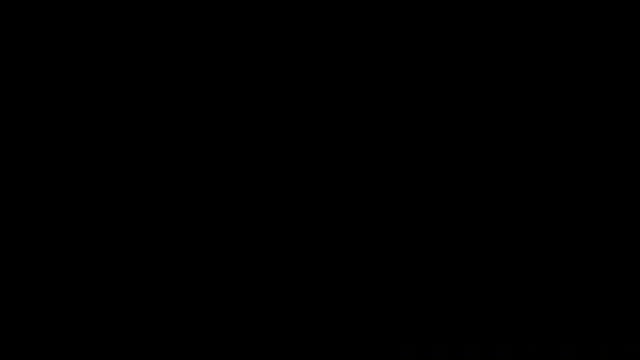 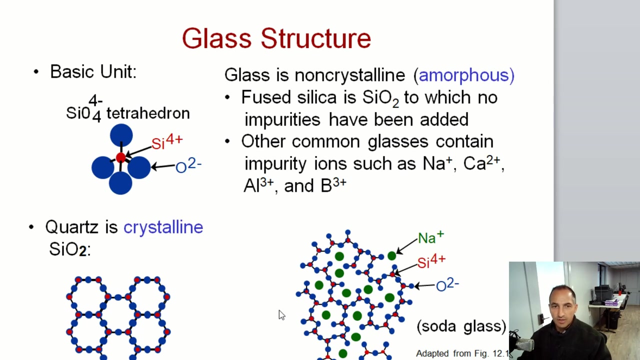 the right is that of the Cristobalite being about Shinonen in Flat. So rocky-doke, So glass structures. The basic unit of the Silicate is SiO4, with a negative charge of four on that and because there is, you know, there's four of. 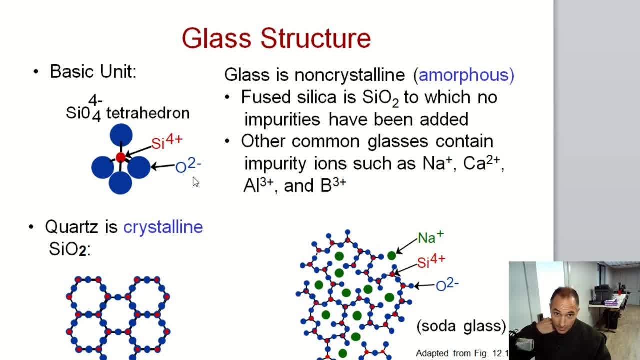 this the oxygens and only one silicon. So the glass is considered a non-crystalline because it's amorphous. However, quartz is crystalline and it has this octahedral type arrangement here of silicon and oxygen. But because of the addition of sodium here we don't have 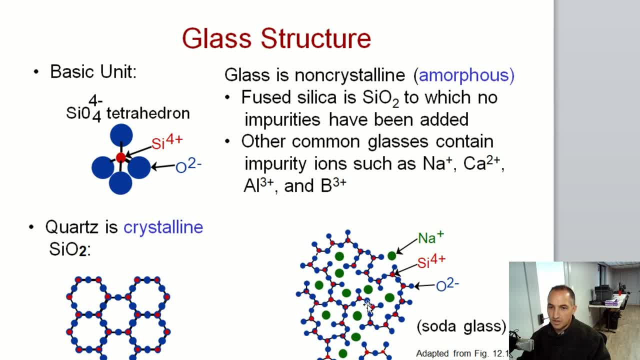 that perfect arrangement. And we can still have charge neutrality with all of these broken bonds in there because of the smaller cation charge of sodium as compared to the silicon. So we can have all these broken bonds and so often add impurities to change the properties. 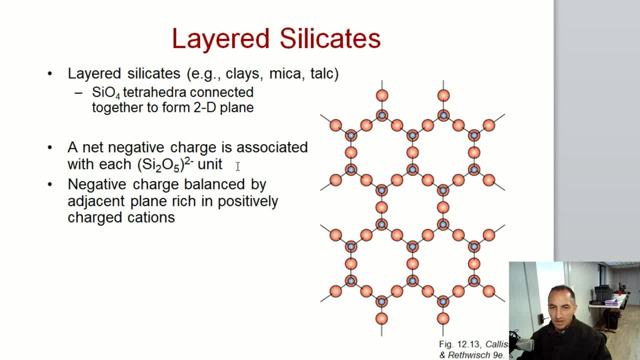 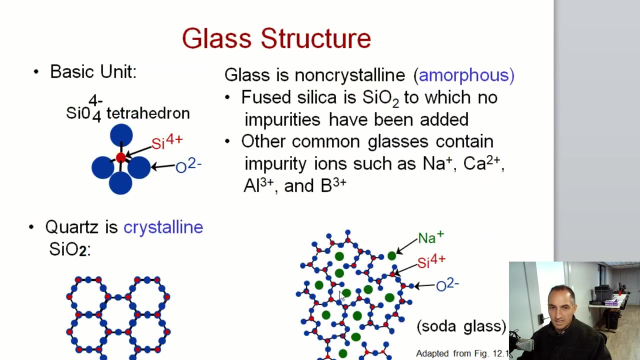 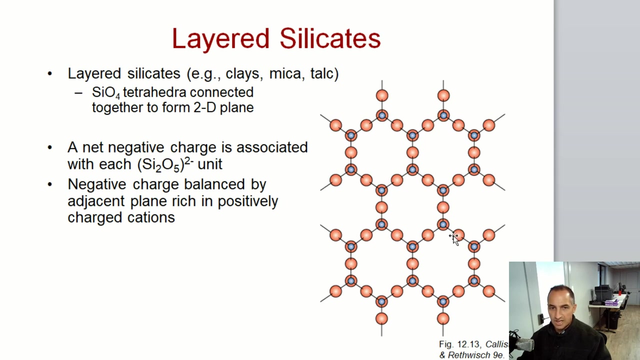 of glasses. There's also something called layered silicates, For example clays, mica, talc. These have these layered structures of the octahedral. They have these layers of octahedral arrangements here and these are just connected together in 2D planes and 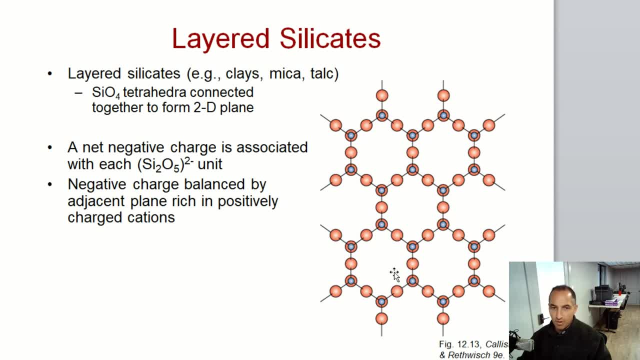 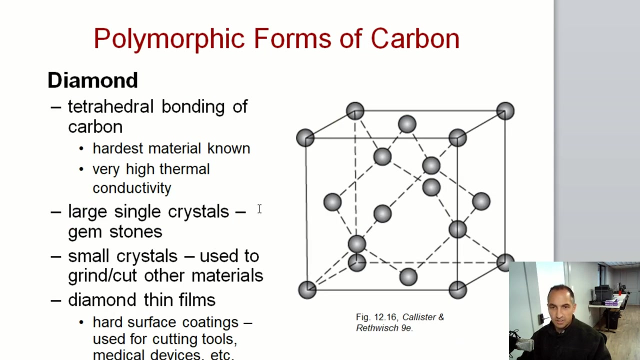 then they're bonded. Adjacent planes are bonded together through weak- like van der Waals- charging between these negative charges that are out of plane right here. So you get negative charging balanced by these charged cations. so polymorphic forms of carbon we're gonna. 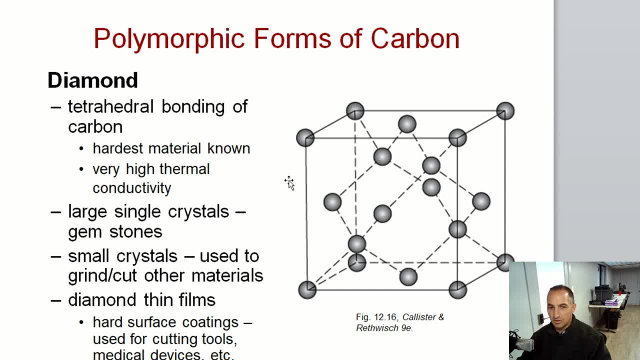 jump into diamond now. diamond doesn't really fit into ceramics, but it's such a unique material that we figured the only place to put it here was in the ceramics chapter. so let's just talk a little bit about it because it's so important. the polymorphic forms of carbon are the tetrahedral bonding carbon there are. 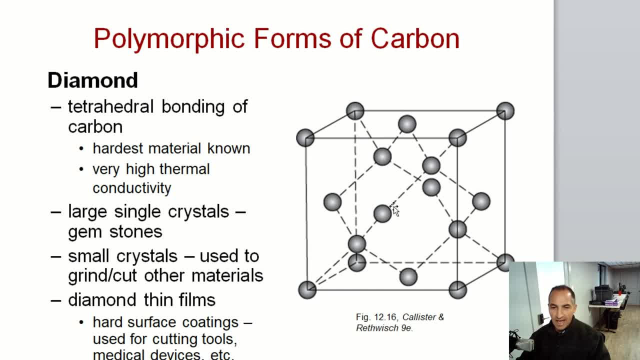 four, four neighboring carbon atoms, and one, two, three and four. you just look at this one here. you have four surrounding it that are bonded to it. it has a large that you can have large single crystals of diamond like gemstones. the small crystals are used for the carbon bonding of the polymorphic forms of carbon. so 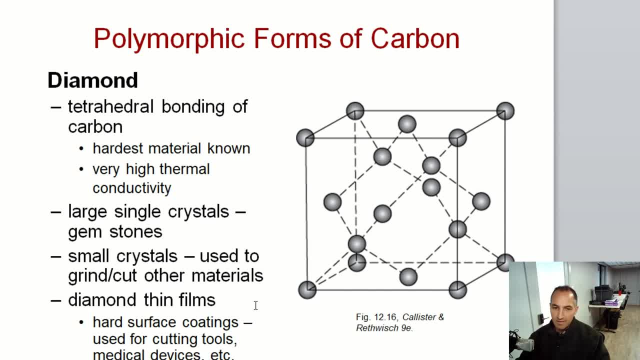 polymorphic forms of carbon are the tetrahedral bonding carbon. there are four for grinding and cutting and you can have diamond thin films that are deposited, that are hard surface coatings and those are cutting tools and medical devices. so carbon is also in, can also be in. 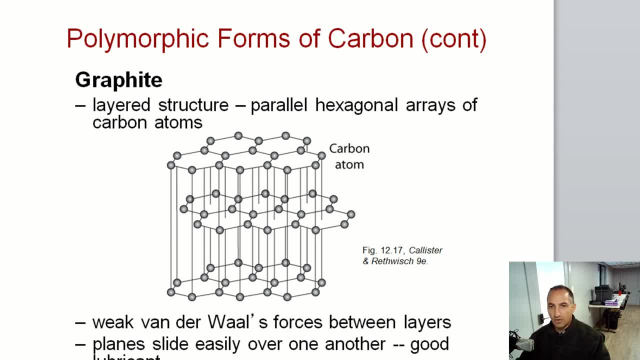 layers instead of in crystalline form, and when carbon is layered, we call that graphite. so graphite is what's used in pencil lead. it's just layers of carbon atoms that are weakly bonded together by these van der Waal forces, and so graphite is actually a very good lubricant, you might. 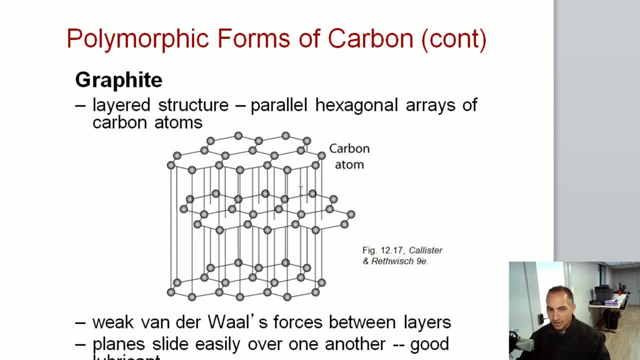 have seen graphite sprays or other things. it's also a constituent in cast iron and the graphite plates made cast iron very machinable because of the lubricating property of graphite. so, and that's again, it's because these graphite plates can slide past each other with the weak van der Waal bonds. 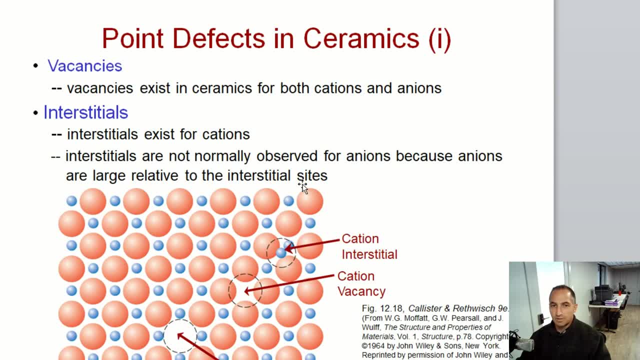 now we're going to jump into point defects in ceramics. so ceramics can either have vacancies or they can have interstitials. vacancies exist in ceramics and they can have interstitials, or they can have interstitials for both cations or anions. so here is an example of a cation vacancy right here. 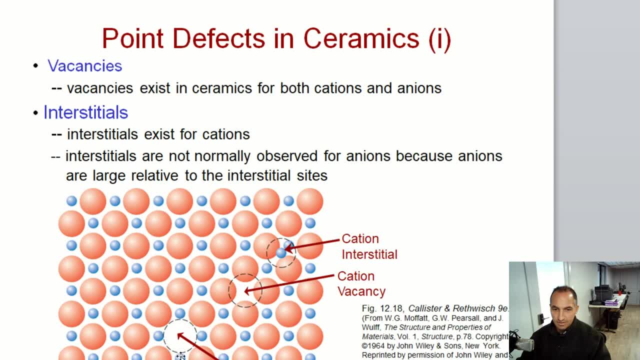 here's an example of an anion vacancy. so you have to have these in pairs to recharge neutrality. if you have a cation vacancy, see. alternatively, you can have an interstitial and an interstitial is just shoved into the lattice as an extra. cations normally doesn't exist for anions because anti ions are much. 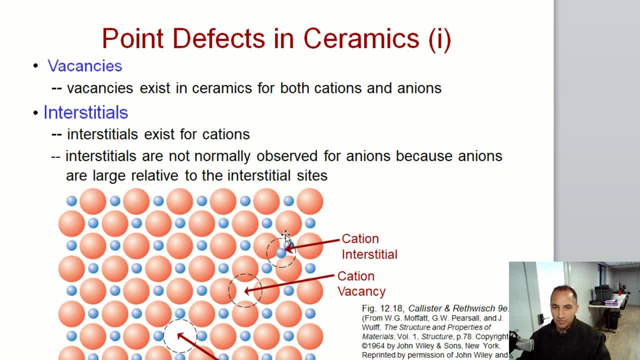 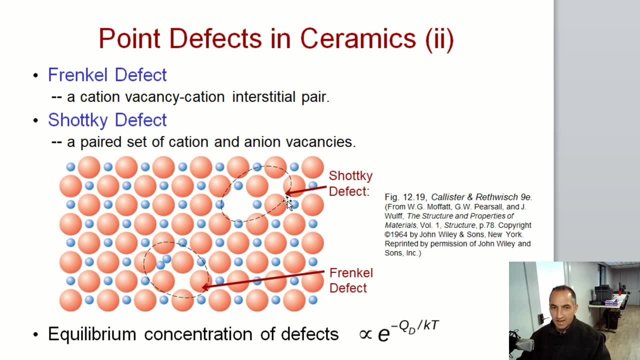 larger and to get in anion interstitials would be difficult to cram into that lattice. so as far as charge neutrality for these defects, there are two types of ceramic defects. there's what we call the, the France defect, and a Schottky brauchen die. 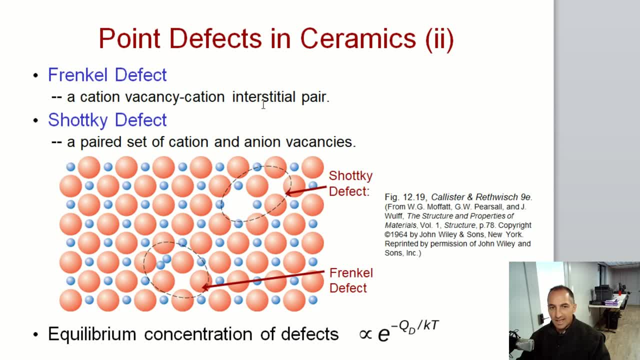 Fraktion Defects. There's what we call that, the Franckl defect and a Schottke Defect. The Frankel defect is a ceramic congo defect. that's where The Frankel Defect Defect and the Schottke defect. 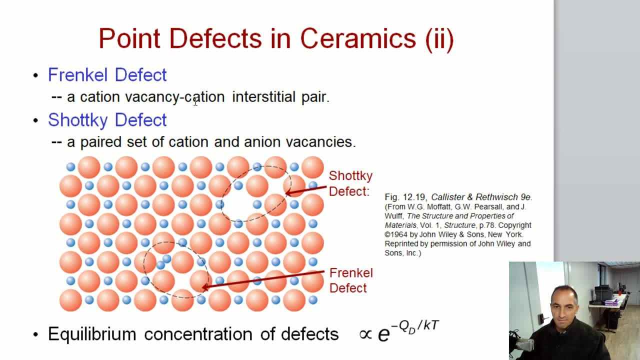 Defect Defect and the Schottke defect is body carbon weight and Junts x этом defect. it's just a cation vacancy cation, interstitial pair. so if you look at what's going on down here, to maintain charge neutrality in the crystal, if you're going to have 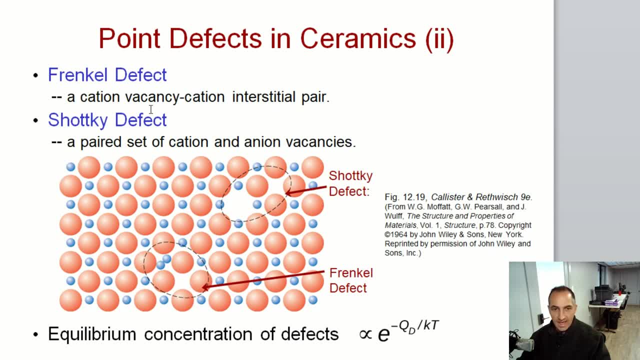 um a yeah, if you're going to have um. well, actually, let me talk first about the shock- you're going to have charge neutrality here. if you're going to have to remove um a cation, you also have to move the like you have removed the cation here, you also have to. 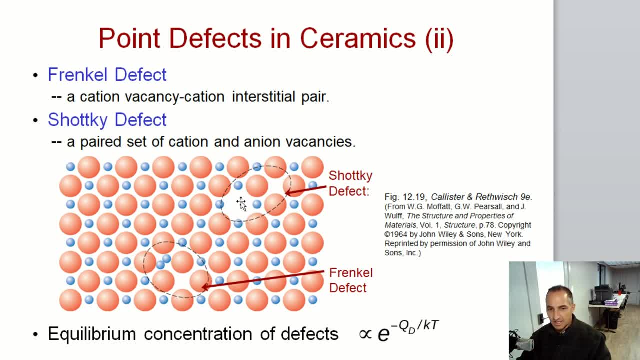 remove the anion here, maintain charge neutrality. so the shot key defect here is charge neutral. a frankl defect, on the other hand, is just um one of the interstitials that's moved out of its site here and it's been rammed into this other site, not really an energy preferred. 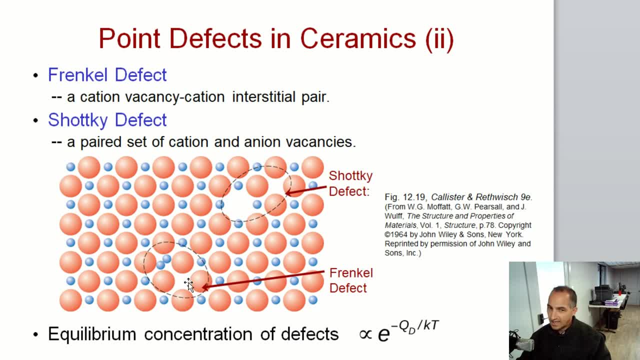 but it's been rammed into this other site and it's been rammed into this other site situation. much rather be here. but in any case, sometimes that interstitial can end up in the wrong place and that's called a frankl, a frankl defect. i like to remember, uh, the shot key defect. 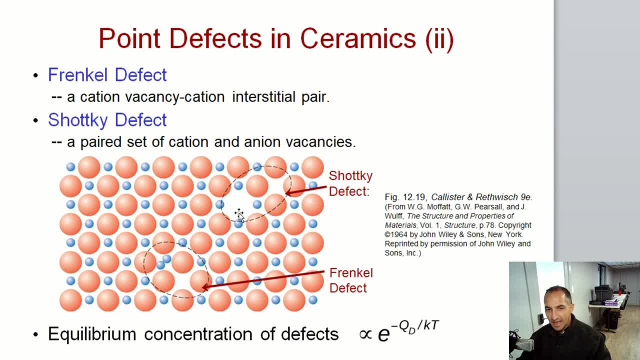 because i think of, like you're. you know you're shooting out atoms from the matrix uh. so, like you know, these guys are being removed. however, in the shot key nothing's being removed, it's just a reposition of an interstitial. so that's the frankl uh defect and the um the equilibrium. 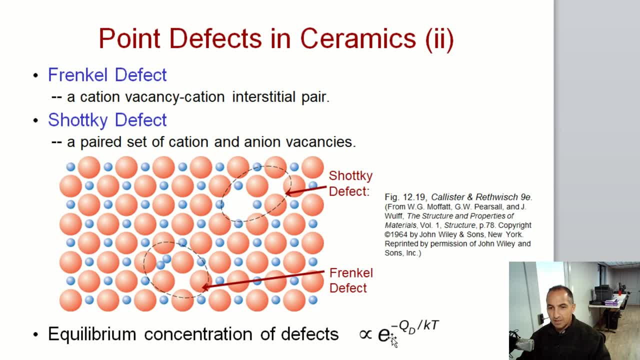 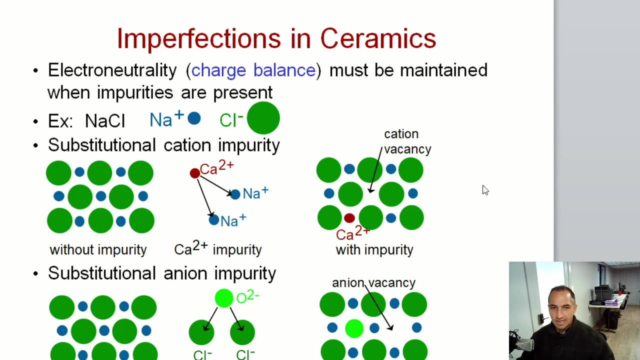 concentration of these defects is related to the um arrhenius relationship which has been brought up before, and so the higher the temperature here, the greater the concentration of these defects, of imperfections in ceramics. and what we can do to maintain uh charge neutrality. uh, let's take for as an example the rock salt or sodium chloride. 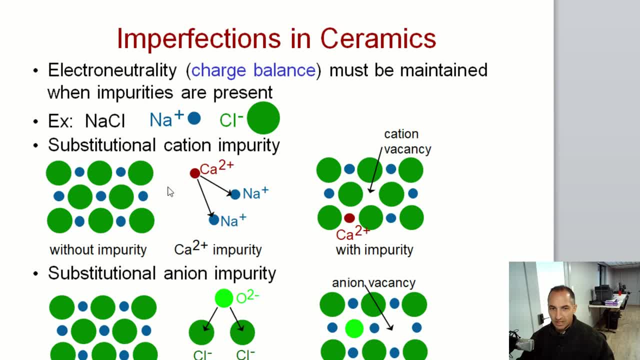 ceramic here and we added an impurity of calcium inside. so in order to maintain chart neutrality, since calcium has a plus two charge, then we have to remove not just the one that's been it being replaced, but an extra one out of the lattice and because sodium is charge as a plus. 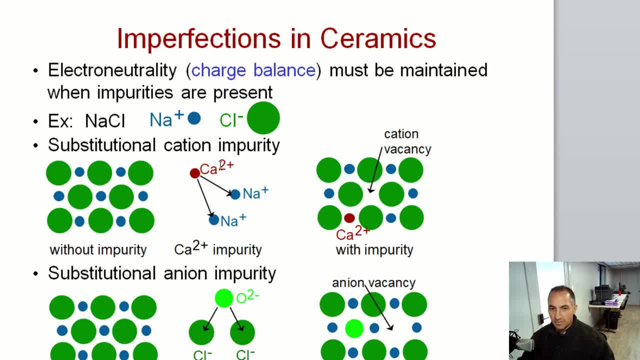 one charge on it. that's why we have to remove two sodiums for one calcium. so we're left with a cation vacancy in the um, substitutional cation impurity. so for um, a substitutional anion impurity. let's say we're going to replace, uh, we're going to put an oxygen impurity into the. 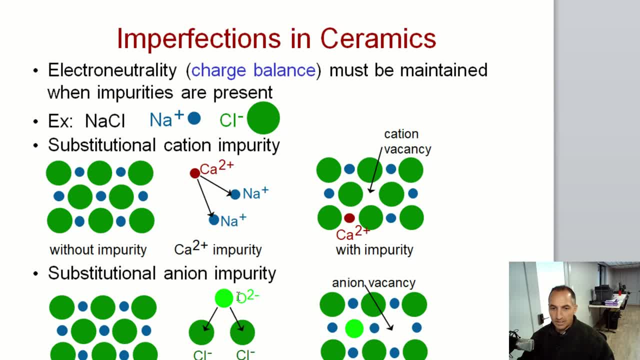 lattice now, but because that has a plus, i'm sorry- a negative two charge, then we have to remove not one of the um chlorines, but two of the chlorines maintain charge neutrality, and so that means we're going to be left with an anion vacancy with a um. 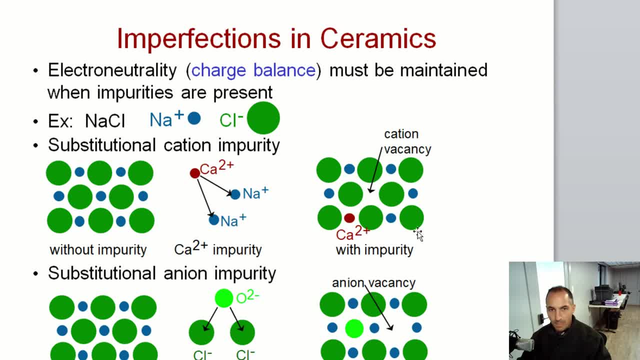 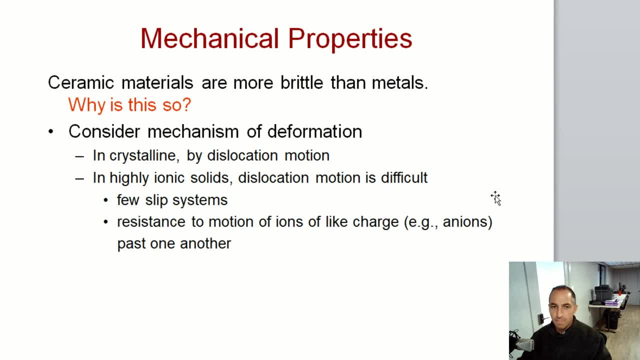 a substitutional anion purity. now let's look at mechanical properties of ceramics, um. so let's um consider what would happen if we tried to just do a regular old tensile test, um, of a ceramic bar. well, it would kind of just shatter everywhere and it would be pretty dangerous. so when we look at mechanical 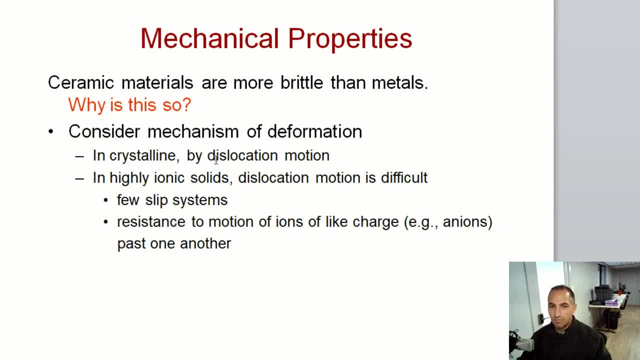 properties, ceramics- we're going to see that it's going to be pretty dangerous. we don't do tensile tests, we do bend tests and um, let's consider the um mechanisms of deformation. so we know that ceramics are very brittle, uh, and when they're in crystalline form, 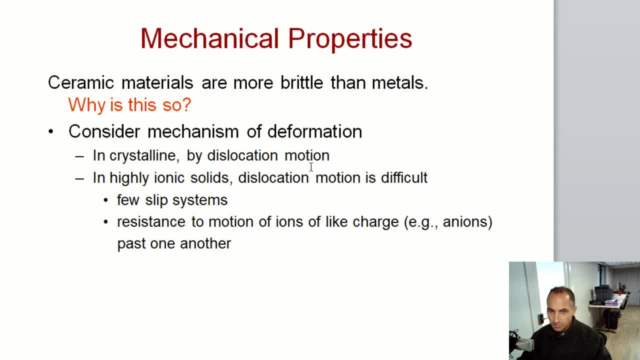 they move by dislocation motion and uh they're um very. you know those dislocations are very difficult to move because of the um ionic nature. you know that there's very few uh slip systems and there's a resistance to the motion because the ions have to slide past each other and sometimes they have to get very close. 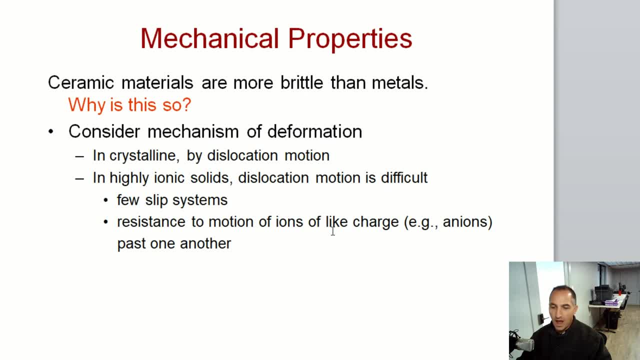 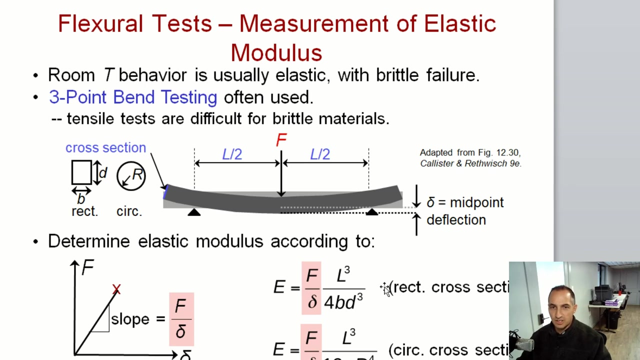 to um ions of their same charge, so they do not like to get very close to each other. as you saw, the um the bonding energy spikes dramatically. you try to get these atoms really close to each other, all right, so. so instead we do these um flexure uh tests and uh kind of like um we did flex tests. 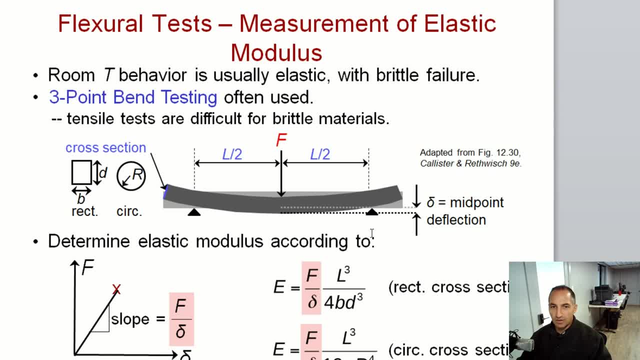 on our aluminum um bars earlier in the quarter. uh, we do these three-point bend tests and uh, we can calculate the elastic modulus through these equations here. the first one is when there's a rectangular cross section, and then the one down here is when you have a cylindrical cross section. so we can get the elastic modulus by um, knowing the um. 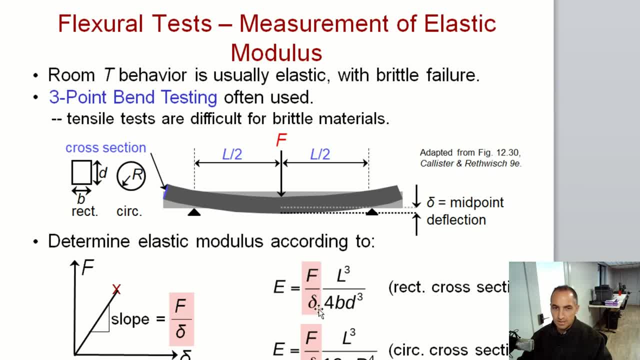 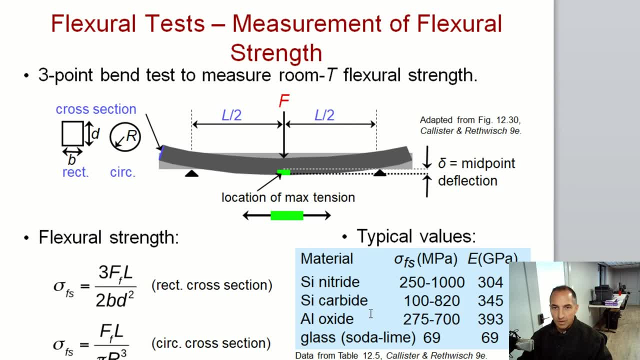 which is just the you know force over the delta, which is the deflection distance. all right, so, um, here is a example, here um typical values for some of these values for elastic modulus of silicon nitride, silicon carbide, aluminum oxide and glass. they're all very, very high, much higher than metals, except for this one and um, the flexor and the. 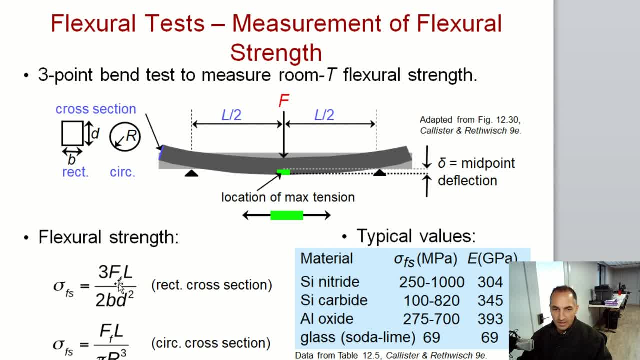 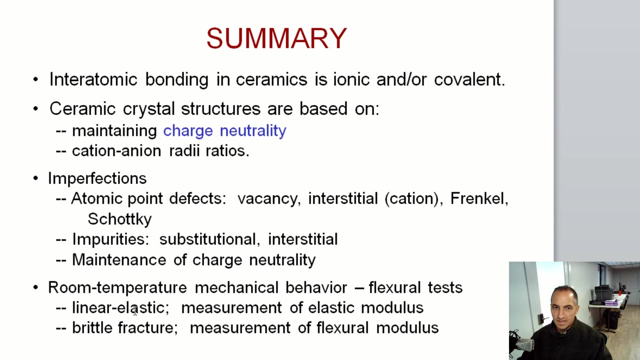 flexor strength and um, calculated using um slightly different equations for rectangular cross section and radius. so we have elastic modulus and the flexor strength, which is sigma sub fs. all right, so in summary, uh, we looked at the interatomic bonding and ceramics and, uh, that bonding is typically either: 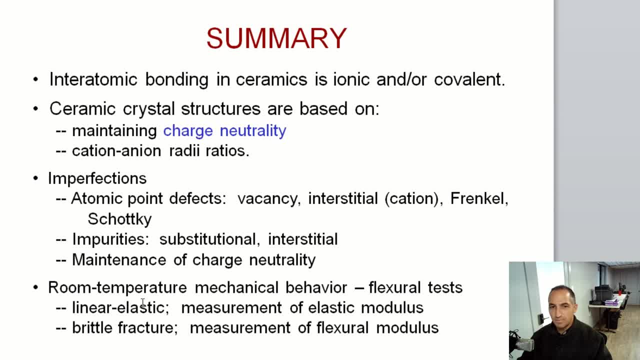 ionic or covalent or a combination of the two, and the crystal structure is going to be dictated on maintaining charge neutrality and the cation to anion radii ratios. so, talking about imperfections, we looked at several different types of imperfections: for defects, there's vacancies, there's interstitial, which are normally cation interstitials looked at. 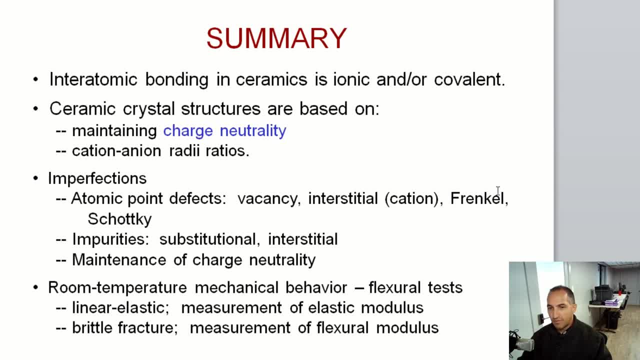 the frankl, which is just a shifting of the anion into another location, and a shot key, which is the removal of both the cation and anion from the lattice. we also looked at impurities. so we looked at the impurities of the cation and anion from the lattice. we also looked at impurities. 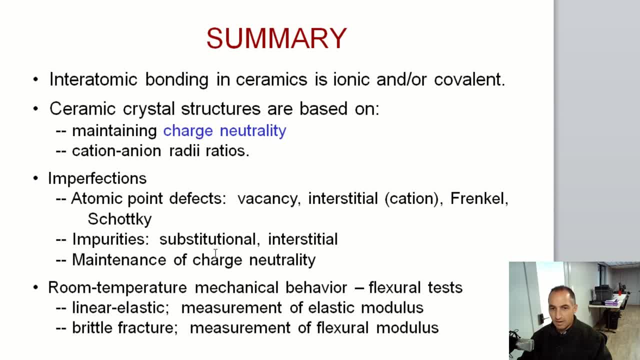 by substituting either an anion or cation. we can go into interstitial sites or substitutional sites and we are always maintaining charge neutrality number. these impurities are Adam. our impurities are added a room temperature. we can do room temperature mechanical tests with ceramics, not tensile tests.